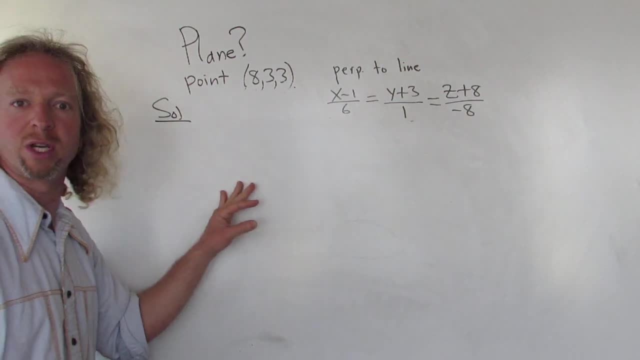 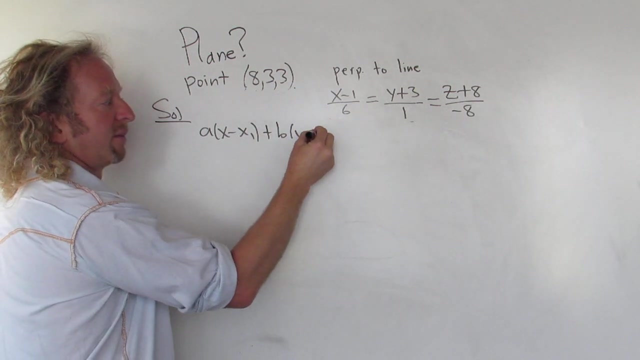 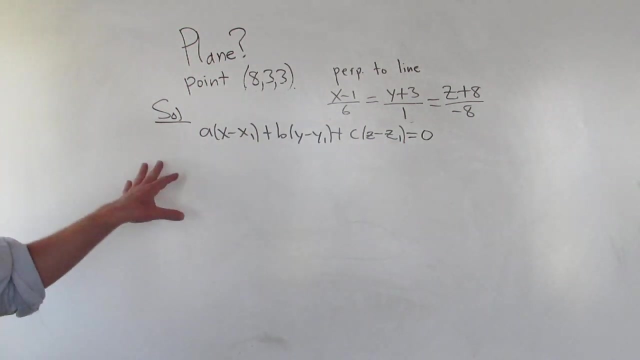 So before we do that, I'm going to go ahead and write down the formula that gives us the equation of the plane. The formula is: a times x minus x1, plus b times y minus y1,, plus c times z minus z1, and all of that is equal to zero In this formula. this is the formula. 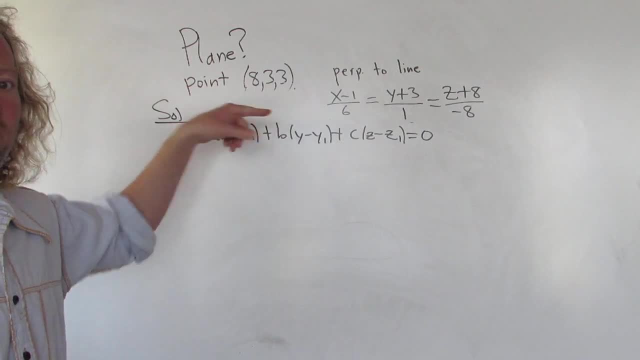 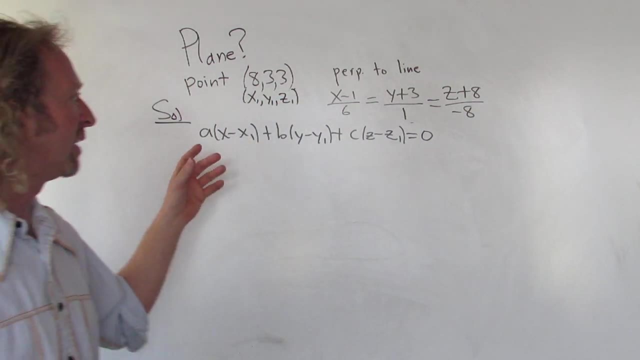 for the equation of a plane. our x1, y1, z1 is a point that lies on our plane. So in this case it's just these numbers here. so really simple. The tricky part is to find a, b, c. 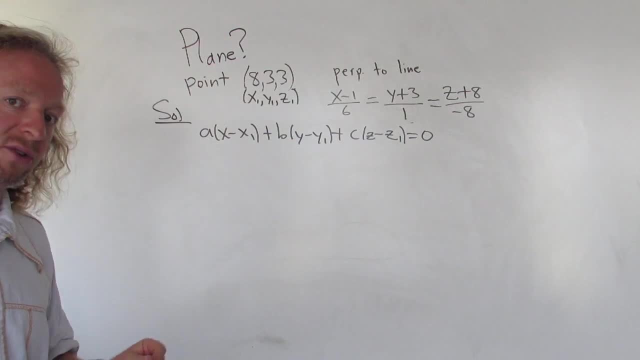 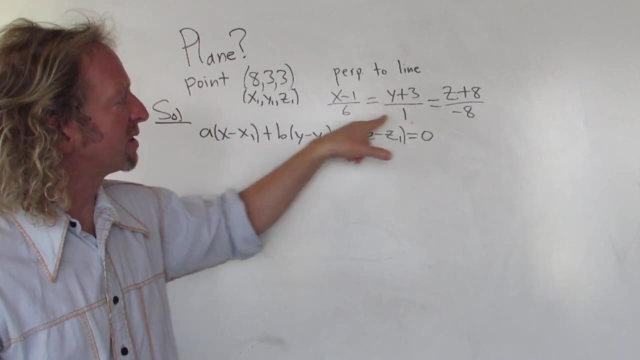 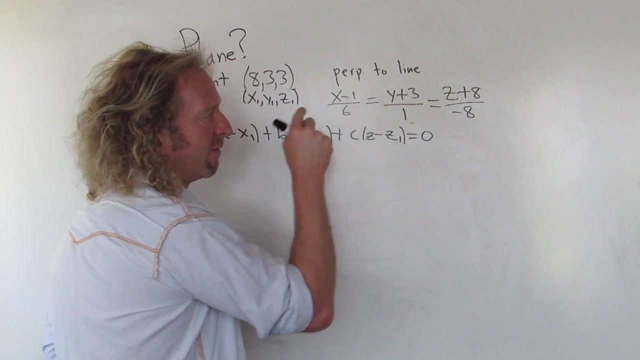 a, b, c are the components for our normal vector. So the vector a, b, c is perpendicular to our plane. Okay, these are the symmetric equations of a line. Okay, if you remember from previous math, the vector that is parallel to this line is: 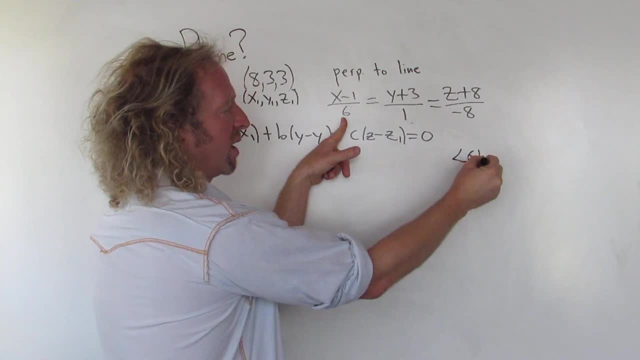 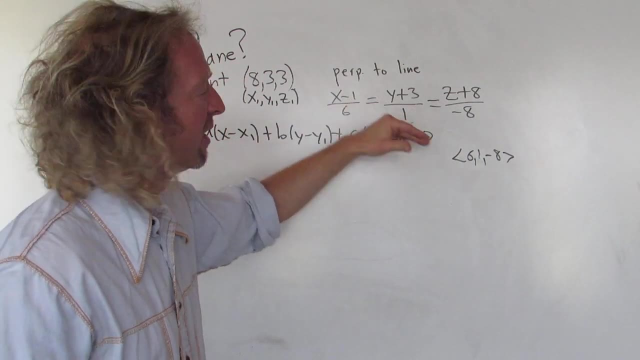 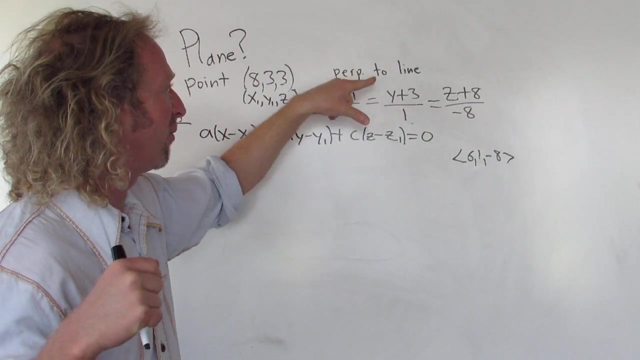 called the direction vector and its components are 6,, 1,, negative, 8.. They come from here. Those are called direction numbers. Okay, so this vector is parallel to this line. Okay, this vector is parallel to this line. Our plane is perpendicular to this line. Therefore, 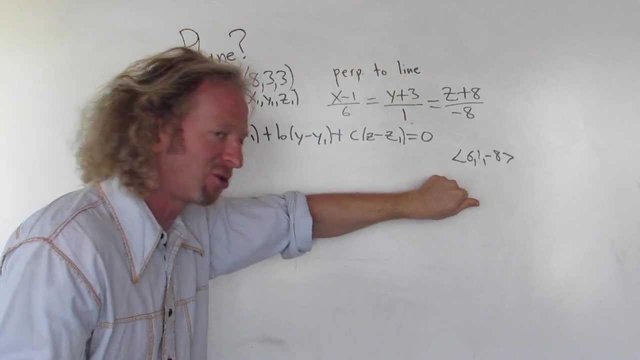 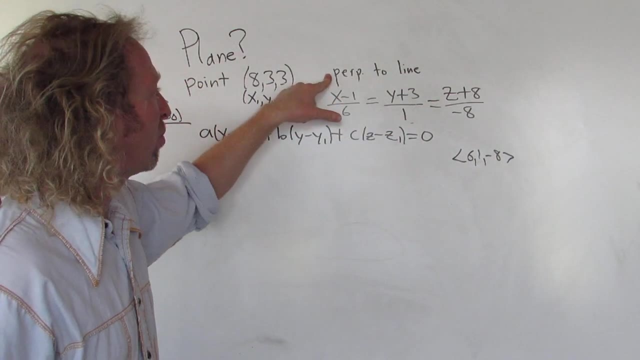 our plane is perpendicular to this vector, so this is the normal vector. Again, this vector is parallel to this line. It's called the direction vector. Our plane is perpendicular to this line. Therefore our plane is perpendicular to this vector because 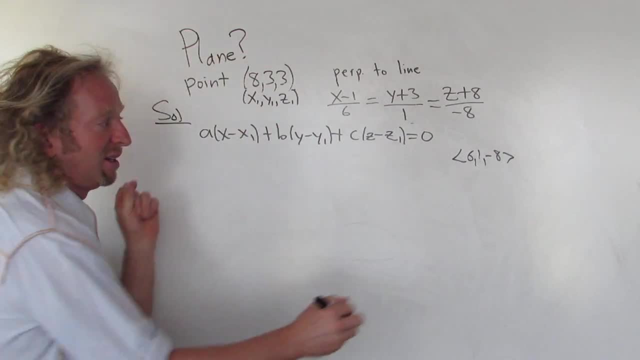 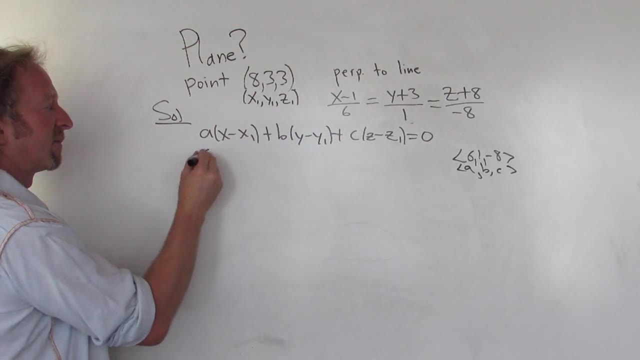 the vector is parallel to the line. So that's our a b c, right, That's our a b c. So a little bit harder, a little bit more thinking there. Let's plug everything in. So a is 6, x minus 8, plus. 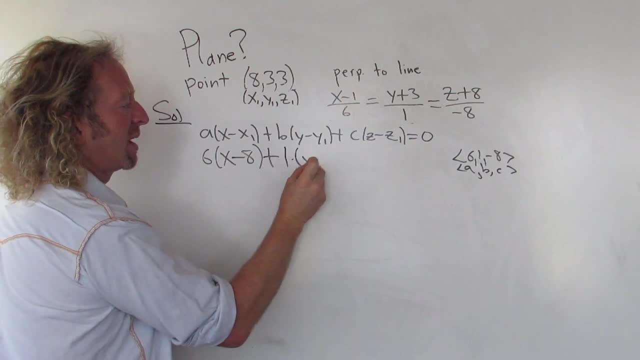 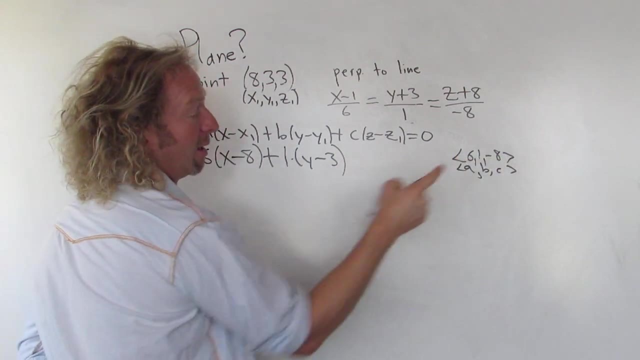 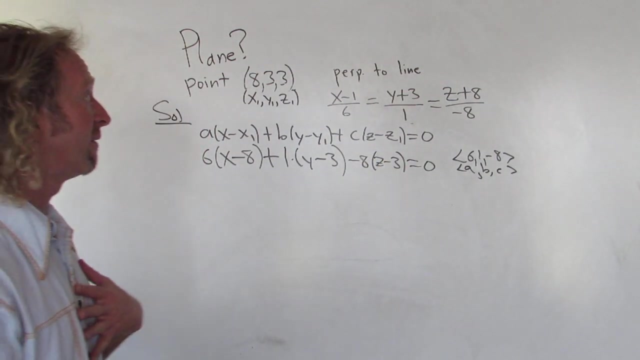 and then b is 1.. That's y minus 3.. And then c is negative 8, right. So looking here, a, b, c, almost messed up. Really easy to mess up on these. Be really careful when you're doing these problems, A common mistake that I have found: 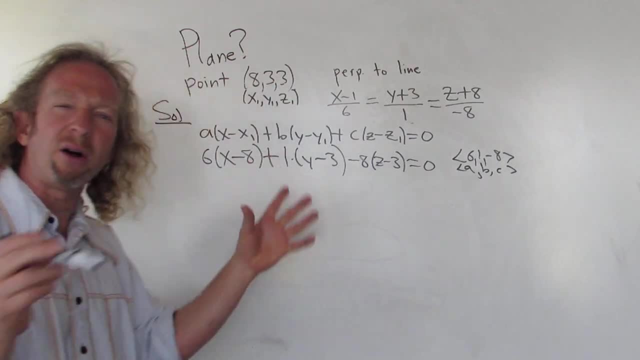 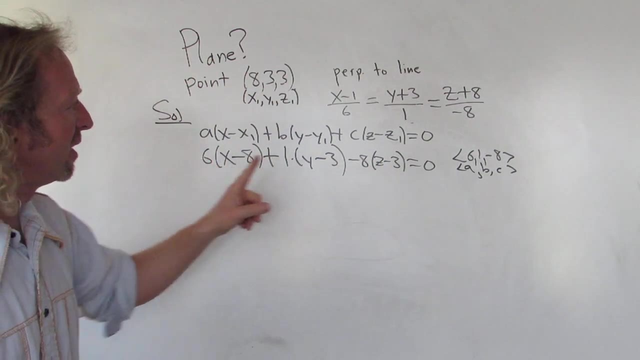 I make myself is just plugging in the wrong numbers, Like you do all the thinking, you write everything down so you understand the problem, but you just make a silly mistake plugging in the numbers. So let's just check that. So a, b, c, that's our vector, that's normal to our plane.